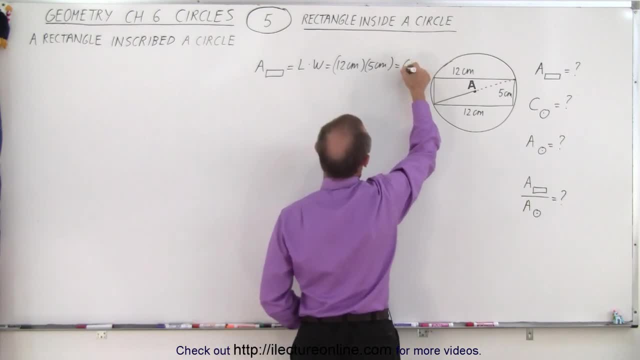 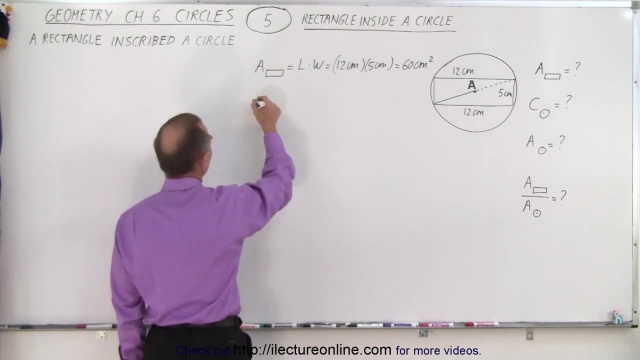 yeah, there's 5 centimeters. So you can see that the area is 60 centimeters square. So that was easy. So now for the circumference. To find the circumference, we'll need to find the diameter. So the diameter squared, which is the hypotenuse, is equal to the sum of the squares of the two sides, So would be 12. 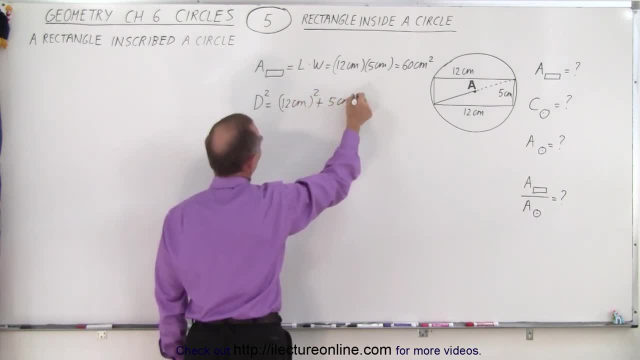 centimeters squared plus 5 centimeters squared, So that's using the Pythagorean theorem. We then say: well, that means that the diameter is equal to the square root. by taking the square root of both sides, I take the square root of this, so it would be 144 centimeters. 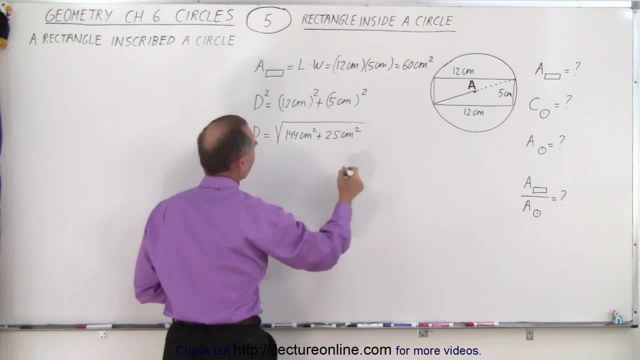 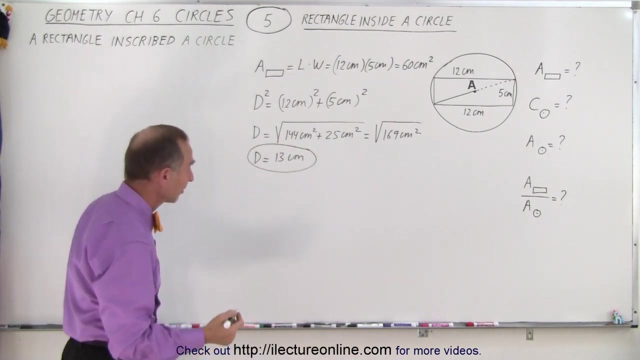 plus 25 centimeters squared. so this is equal to the square root of 169 centimeters squared. and then we take the square root of that, we get 13 centimeters. so now we know that the diameter of the circle is 13 centimeters, and since the circumference is equal to pi times the diameter, that is equal to. 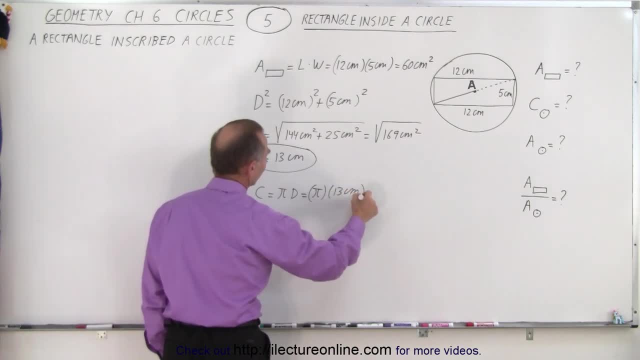 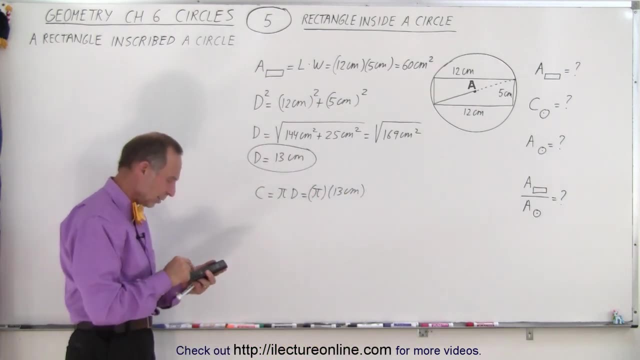 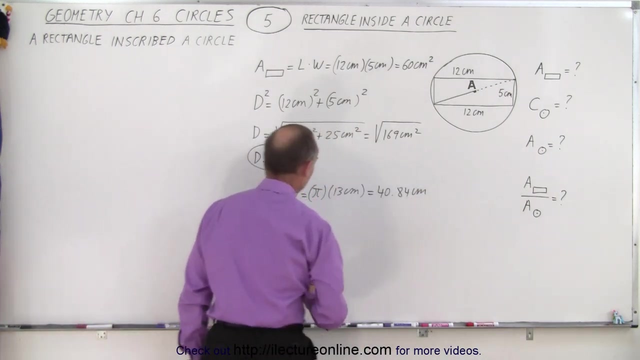 pi times 13 centimeters, of course, pi is 3.14159, none and none and none. but if you have a calculator, you just simply take 13 times the number pi and you get 40.84 centimeters. likewise to find the area of the circle, and I should probably 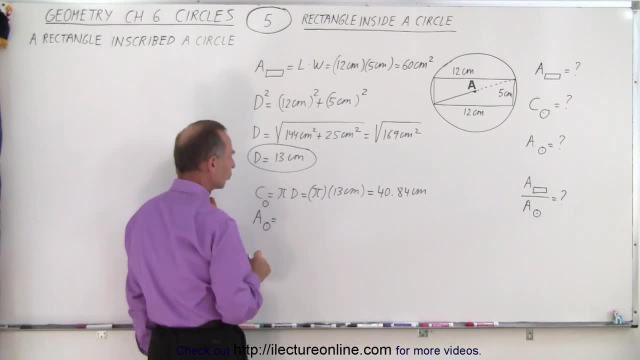 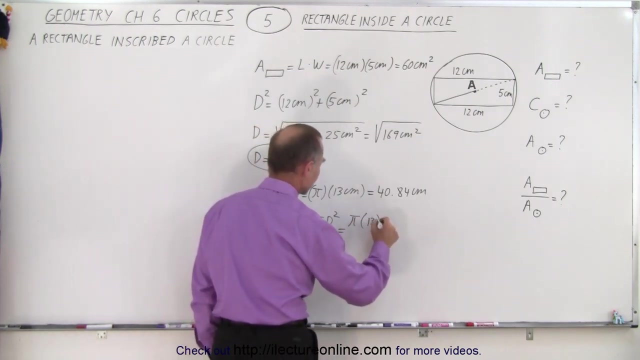 should make a circle symbol, so it is for the circle that is equal to pi R squared, or pi D squared over 4, since we know the diameter will use that. so that would be pi times 13 squared divided by 4, which is equal to pi times 169 divided by 4. so now grabbing. 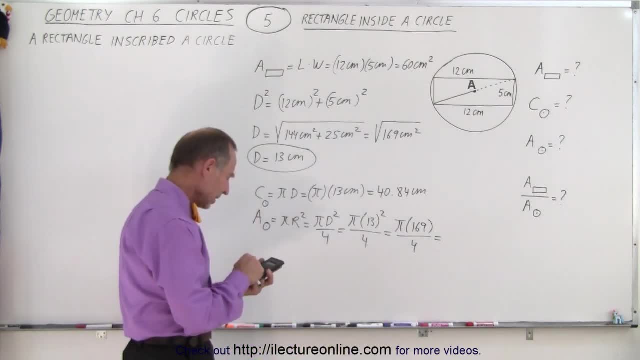 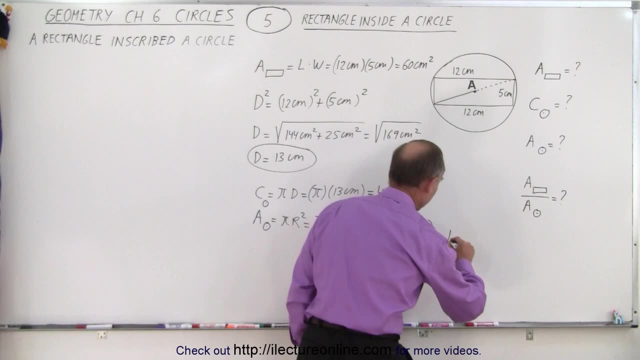 a calculator. we take 169 divided by 4 times pi and we get 132 point 7. that is 132 point 7. that is 132 point 7. that is 132 point 7, centimeter squared, because we're looking for the area. and then 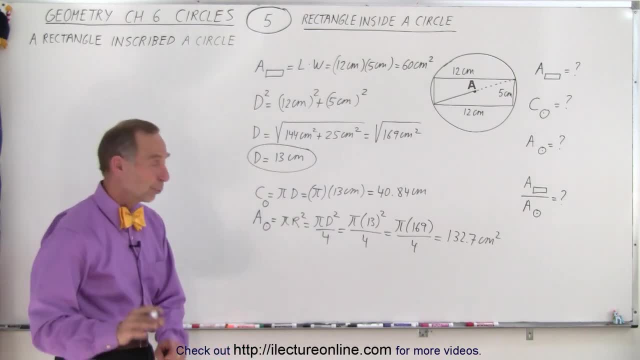 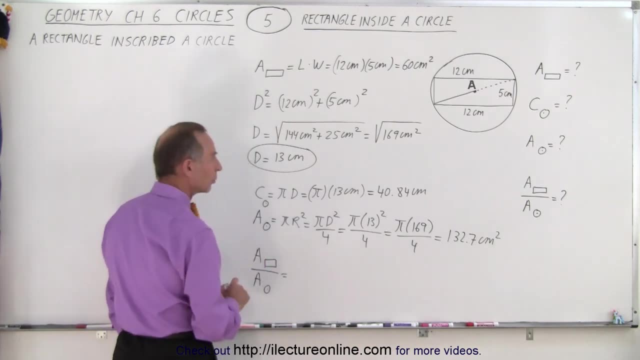 that is 132 point 7 centimeter squared, because we're looking for the area and finally we'll get the ratio of those two. so the area of the rectangle divided by the area of the circle, that is equal to 60 centimeters squared divided by 132.7.